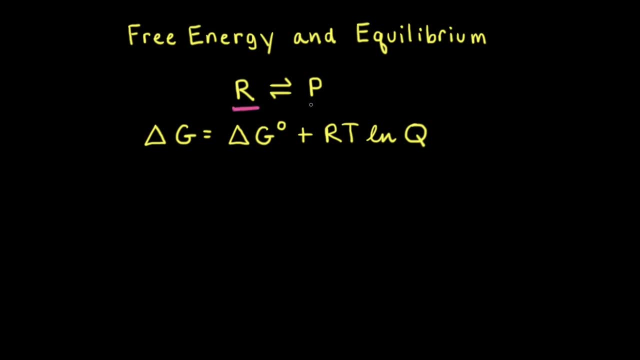 Let's say we have a generic reaction where reactants turn into products, and our goal is to think about the relationship between free energy and this reaction when it comes to equilibrium, First, we need to consider the equation that allows us to calculate nonstandard changes. 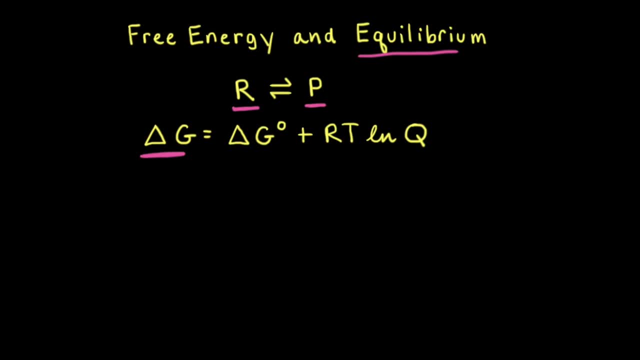 in free energy, delta G. We can think about delta G as the instantaneous difference in free energy between reactants and products, And from the equation we see that delta G is equal to delta G naught plus RT. natural log of Q. Delta G naught is the standard change in free energy. 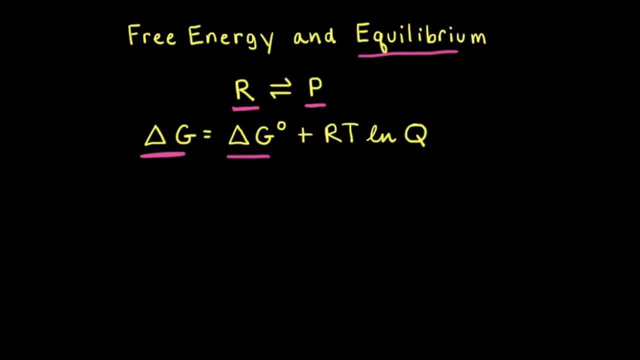 between reactants and products. This value refers to the difference in free energy between reactants and products in their standard states at a specified temperature. R is the ideal gas constant, T is the absolute temperature in Kelvin and Q is the reaction quotient. 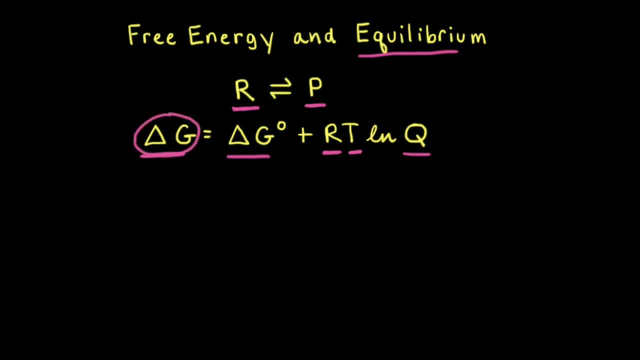 At equilibrium the instantaneous difference in free energy between reactants and products is zero, which means there's no more driving force for the reaction. And at equilibrium the reaction quotient Q is equal to the equilibrium constant K, So we can plug in zero for delta G in our equation. 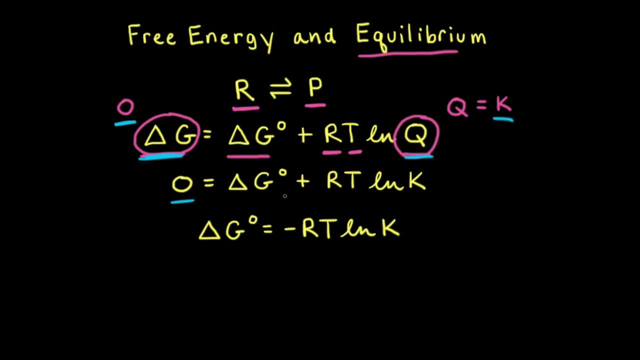 and we can plug in K for Q. That gives us zero is equal to delta G naught plus RT natural log of K. If we subtract RT natural log of K from both sides, we get delta G naught is equal to negative RT natural log of K. 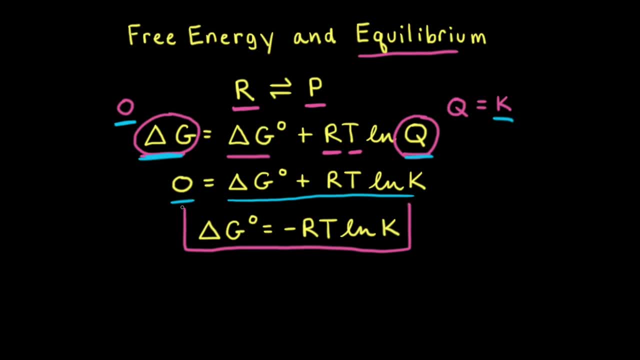 This equation is extremely useful because now we have a relationship between free energy and equilibrium. If we know the standard change in free energy for a particular reaction at a particular temperature, we can calculate the equilibrium constant for that reaction. Next, let's go ahead and go through the math. 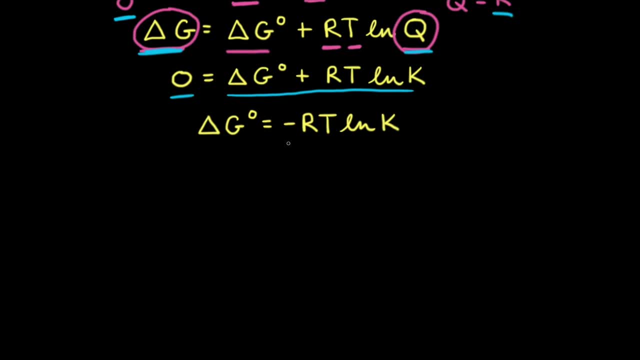 to solve for the equilibrium constant K. To solve for K we need to first divide both sides by negative RT. So on the right side negative RT would cancel out. We could then rewrite it as natural log of K is equal to negative delta G naught divided by RT. 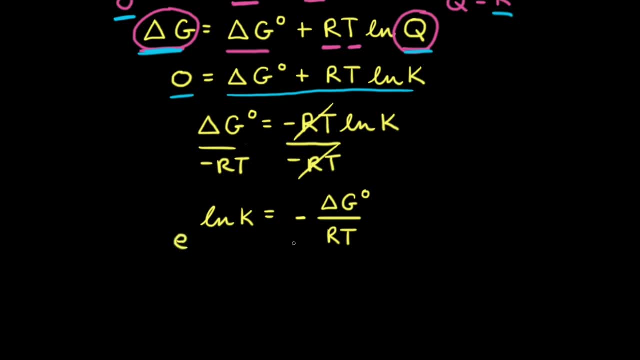 And to get rid of the natural log, we need to take E to both sides, which gives us the following equation: The equilibrium constant K is equal to E to the negative delta G naught divided by RT. So if we know the value for delta G naught, 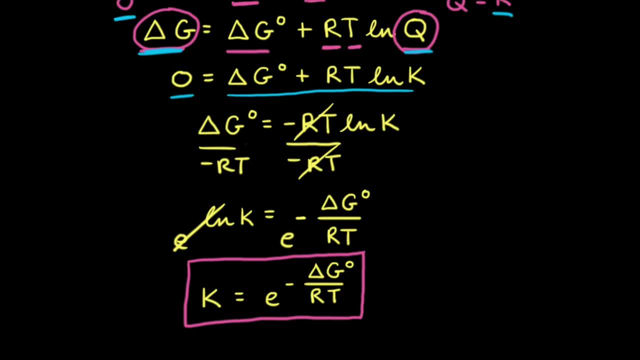 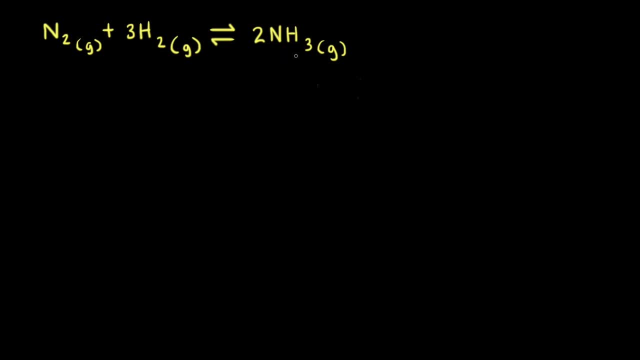 for a particular reaction and we know the temperature, we can calculate the equilibrium constant for that reaction at that particular temperature. Let's calculate the equilibrium constant K for the synthesis of ammonia from nitrogen and hydrogen, And let's do this for three different temperatures. 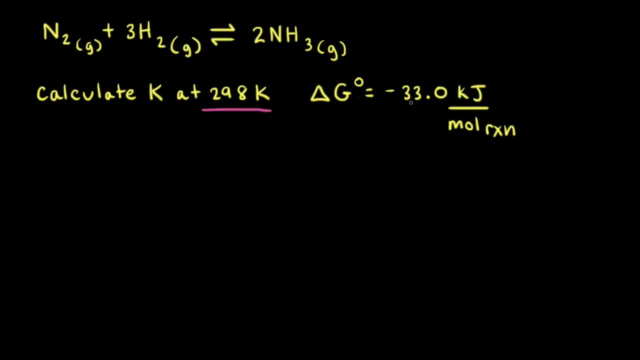 Let's start with a temperature of 298 Kelvin. Delta G naught at this temperature is equal to negative 33.0.. kilojoules per mole of reaction. So to solve for the equilibrium constant K we need to plug in the value for delta G naught. 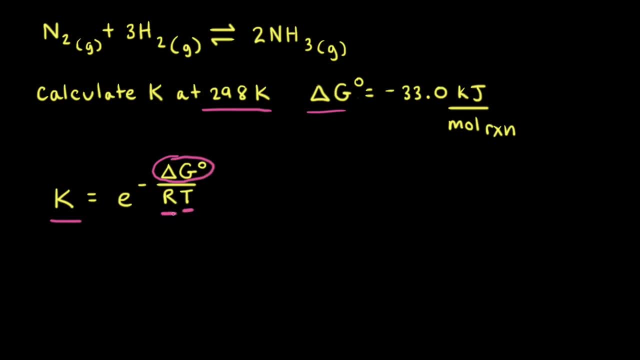 We also need to plug in the temperature in Kelvin and the ideal gas constant R. The ideal gas constant is equal to 8.314 joules per mole of reaction Kelvin And since we're using joules in the units, we need to make sure to convert the units for delta G naught. 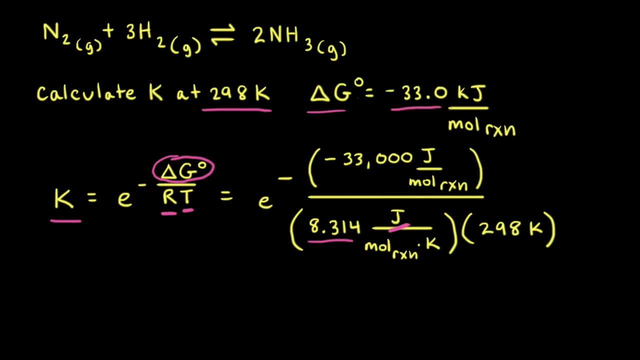 into joules per mole of reaction. So negative 33.0 kilojoules per mole of reaction is equal to negative 33,000 joules per mole of reaction, still with three significant digits And once we plug in our temperature of 298 Kelvin. 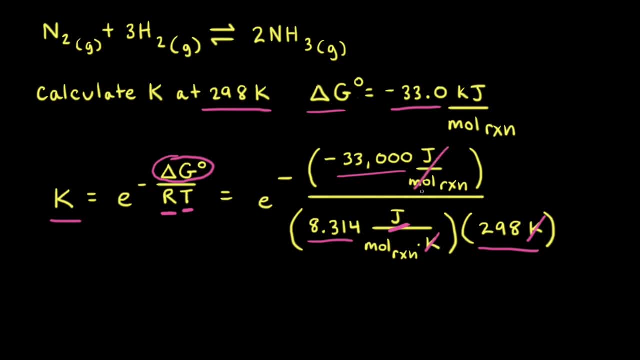 notice how Kelvin cancels out and also joules per mole of reaction cancels out. When we do the math we find that the equilibrium constant K is equal to E to the 13.3 power, which is equal to six times 10 to the fifth. 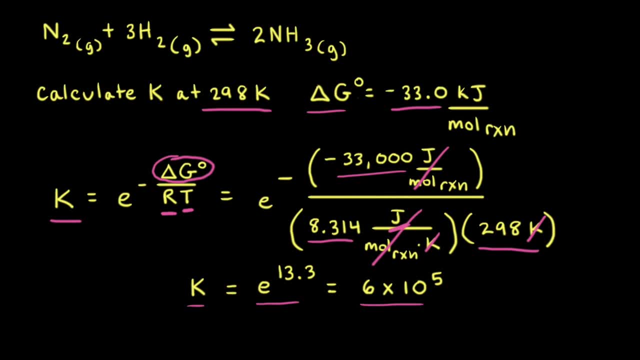 Notice how equilibrium constants don't have units. When E is raised to a power, the result has the same number of significant figures as there are decimal places in the power. Since we have only one decimal place in this power, we have one significant figure for our final answer. 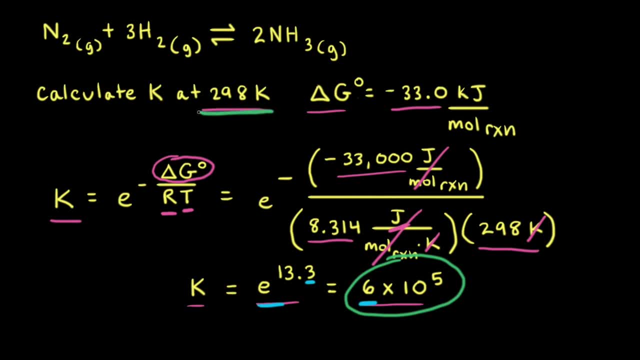 Since the value for K for this reaction at 298 Kelvin is much greater than one, that tells us, at equilibrium there are more products than there are reactants. There's a lot more ammonia than there is nitrogen or hydrogen when this reaction reaches equilibrium at 298 Kelvin. 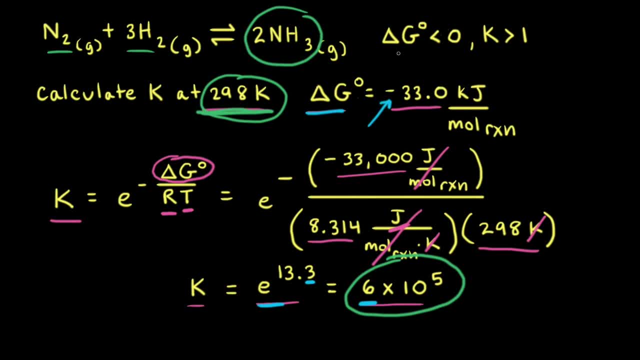 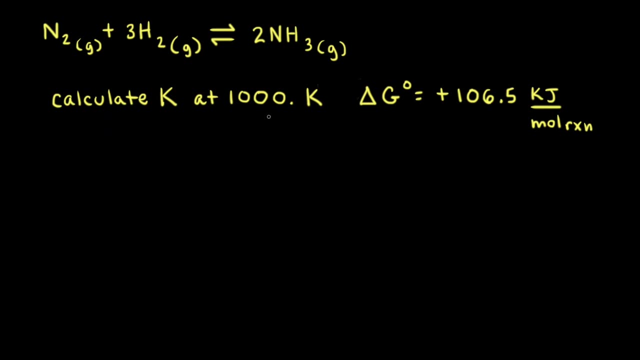 So whenever delta G naught is negative, or you could say delta G naught is less than zero, the equilibrium constant is greater than one and products are favored over reactants at equilibrium For the same reaction. for the synthesis of ammonia, let's calculate the equilibrium constant K. 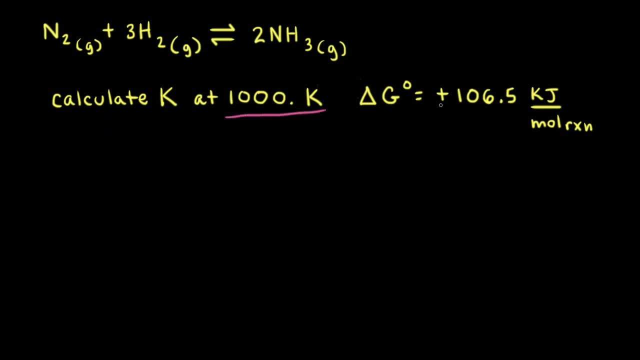 at a different temperature. This time it's 1,000 Kelvin- And at 1,000 Kelvin, delta G naught for this reaction is equal to positive 106.5 kilojoules per mole of reaction, Just like the previous example. 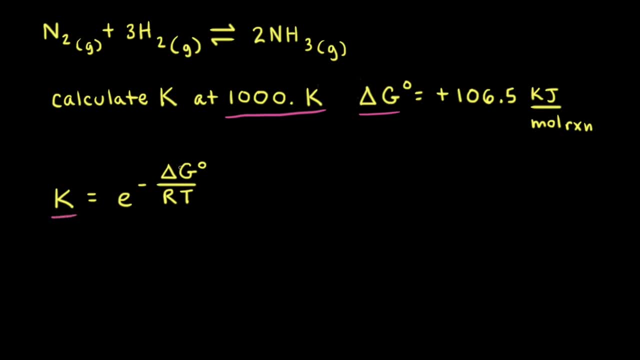 we're gonna plug everything into our equation to calculate K, So we need to plug in delta G, naught, the temperature, which is 1,000 Kelvin this time, and the ideal gas constant, So we plug in the ideal gas constant. 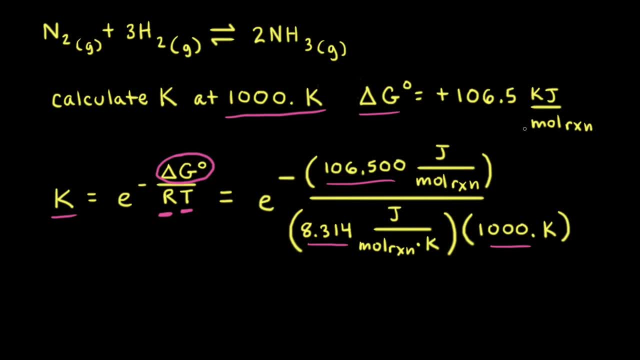 the temperature and delta G naught. Once again we had to convert from kilojoules per mole into joules per mole of reaction. So joules per mole of reaction cancels out and Kelvin cancels out. That gives us K is equal to E, to the negative 12.81 power. 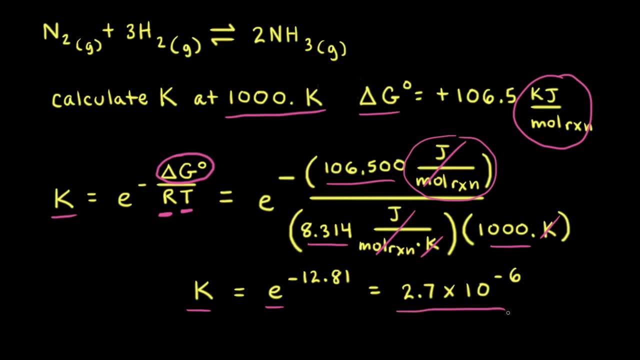 which is equal to 2.7 times 10, to the negative six, Because we have two decimal places in the power, the final answer is to two significant figures. For this example, K is much less than one, which tells us at equilibrium. 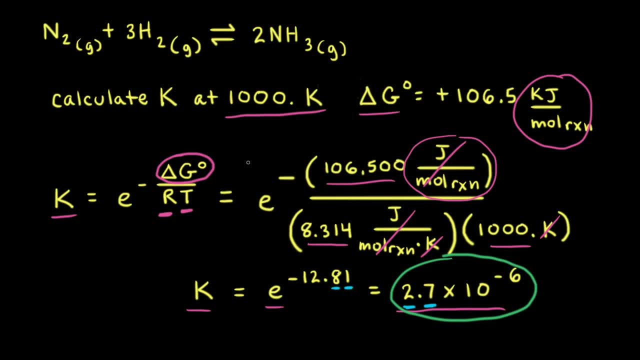 there are far more reactants than there are products. So, at 1,000 Kelvin, if this reaction were at equilibrium, we'd have a lot more of our reactants, nitrogen and hydrogen, and only a small amount of our product, ammonia. 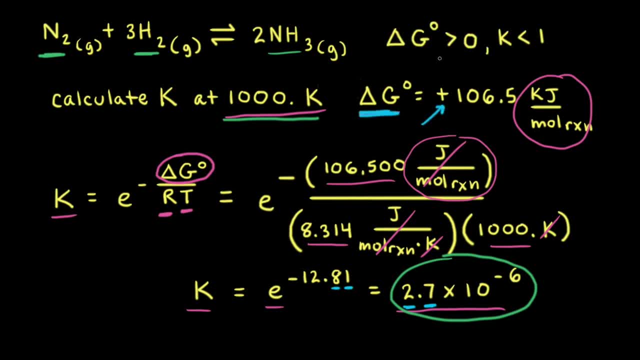 So whenever delta G naught is positive, or you could say delta G naught is greater than zero, the equilibrium constant K is less than one. which means that equilibrium there are a lot more reactants than there are products. And for our last example, 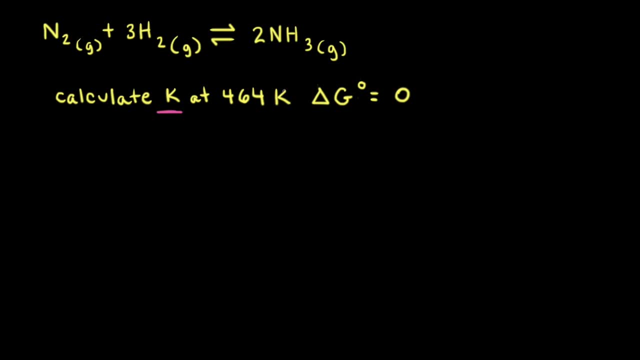 let's calculate the equilibrium constant K for the same reaction, this time at 464 Kelvin. At that temperature, delta G naught for this reaction is equal to zero. Calculating K is a lot easier for this example because if we plug in zero for delta G naught. 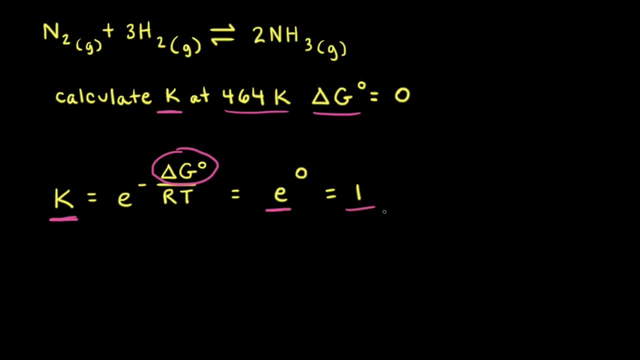 K is equal to E, to the zero power, which is equal to one, And when the equilibrium constant is equal to one, that means that equilibrium there's significant amounts of both reactants and products. So if this reaction were to reach equilibrium at 464 Kelvin,